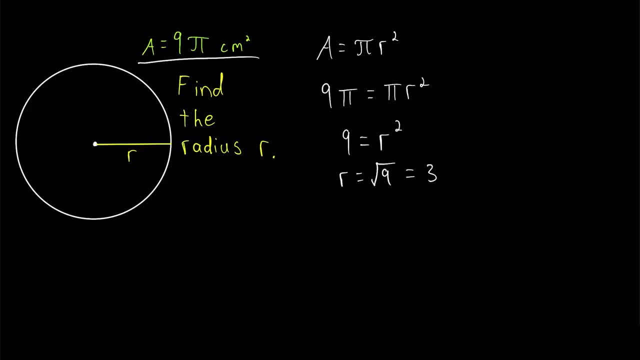 which of course is 3.. And if our area was given in centimeters squared, the radius is going to be the square root of that unit. So the square root of centimeters squared, that's centimeters. Sometimes the numbers will be a little messier, so let's quickly do an example like that. 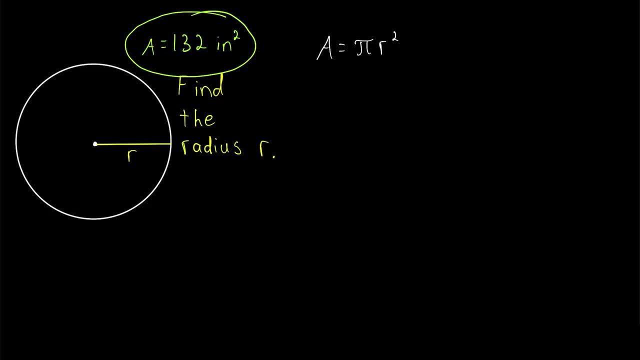 Now the area of our circle is 132 square inches. We again want to find the radius r. It's the same process. Plug that area into the area formula. So we have 132 equals pi r squared, And remember we can leave the units out of the calculation. So we have 132 equals pi r squared, And remember. 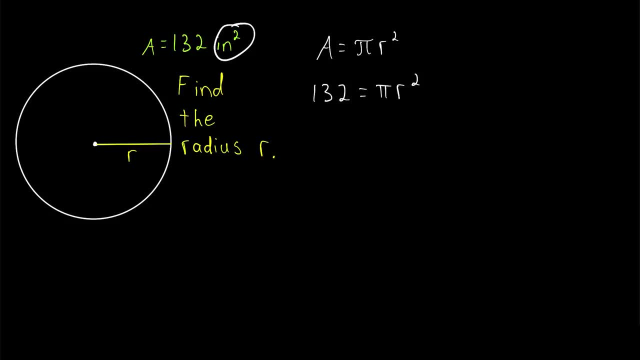 we can leave the units out of the calculation. So we have 132 equals pi r squared. And remember until the end. we know our final unit will be inches. To get to the answer, we just have to solve this equation. for r Again, we'll begin by dividing both sides by pi. That will give us 132. 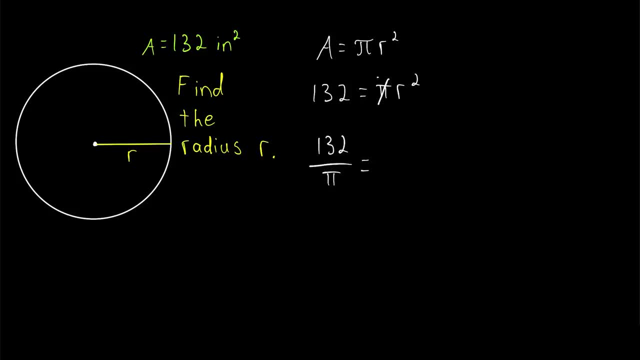 over pi on the left is equal to on the right, the pi will be canceled out and we'll be left with r squared. Then, to finish solving for r, we just take the square root of both sides. That will give us that the radius of our circle r is the square root of both sides. So we have 132 over pi. 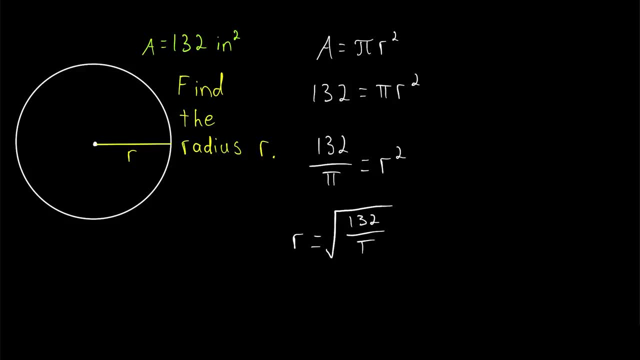 square root of 132 over pi. I've pasted that answer in yellow up here. You might be asked to round your answer to the nearest hundredth, for example. If so, at this point you can just plug that into a calculator and round. Rounding that to the nearest hundredth gives us 6.48 inches. 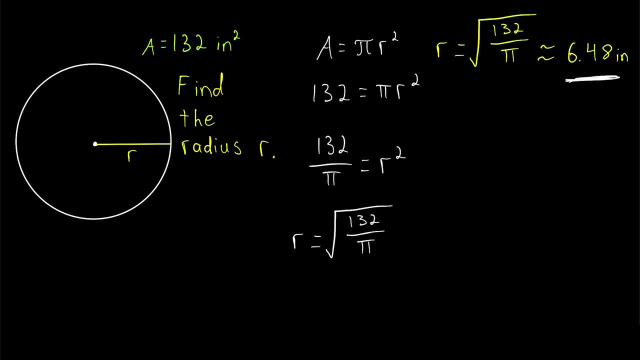 On the other hand, if you're not told to approximate your answer, then you may be expected to leave it in this order. So we're going to leave it in this order. So we're going to leave it in this order exact form, in which case you'll probably want to simplify it. To simplify a radical like this: 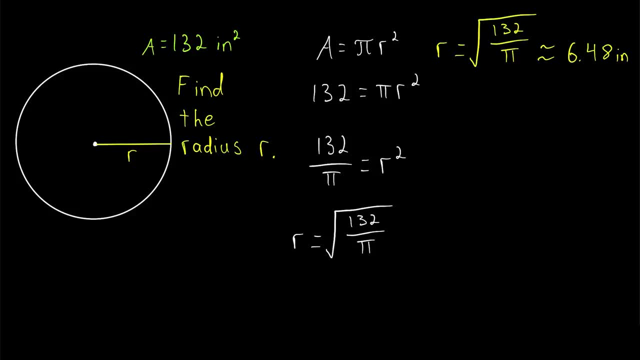 we just want to take out any perfect square factors that we can. So, for example, in this case, 132, we can rewrite as 4 times 33.. So this is equal to the square root of 4 times 33 over pi.